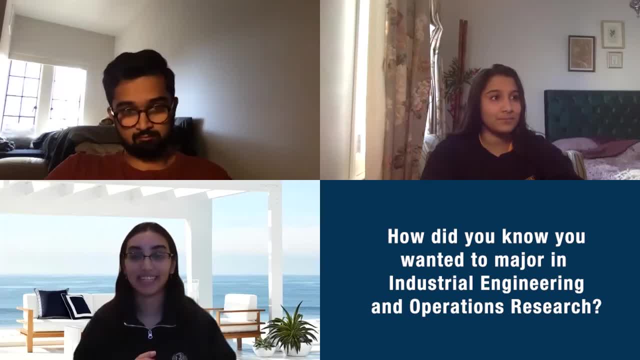 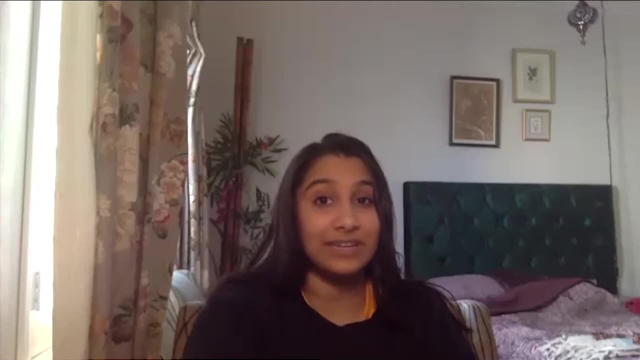 maintenance, scheduling and things of the sort. so I kind of like the idea that it's kind of putting everything together, this big picture. That's probably when I kind of thought: you know, this sounds like the major for me. That's awesome. What projects, internships or research have you guys done that's related to IEOR? 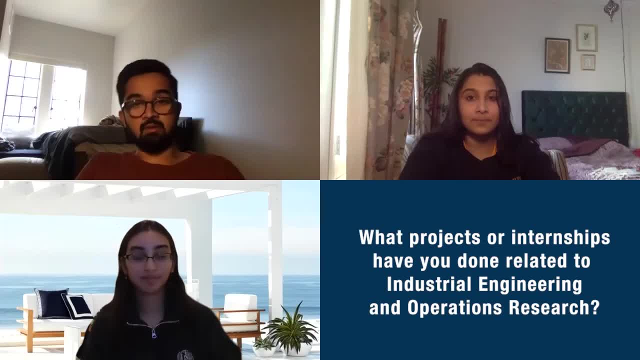 Last summer I did consulting at McKinsey, which is definitely very much related to IEOR. so we were actually doing like IT strategy and helping a company decide, like which you know- which database system to choose and like what were the right choices to make, and so I actually applied a lot. 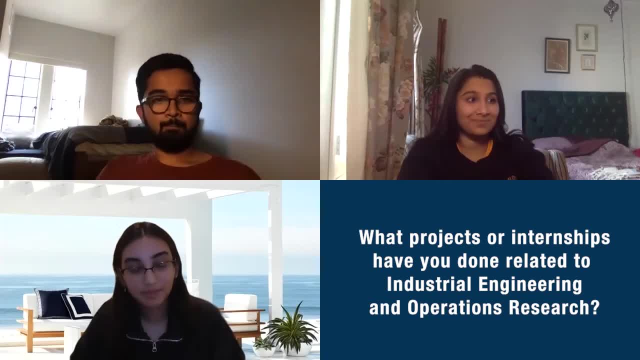 of this one IEOR class, So I think that was really inspiring to me. I think that's something that I really liked about that internship. So that's awesome, And you, Anika. The internship I have done was actually a SWE internship and it kind of really led me into the ML space. so 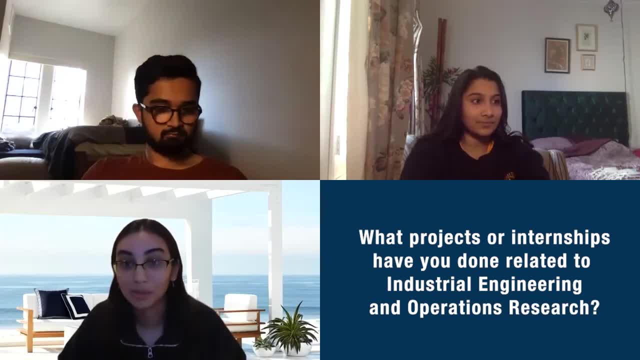 machine learning where there's a lot of optimization that comes into play. So a lot of the algorithms that we'll see people using in CS are things that were really developed in the IEOR space in kind of optimizing and finding these best algorithms. And then I guess on my experience. 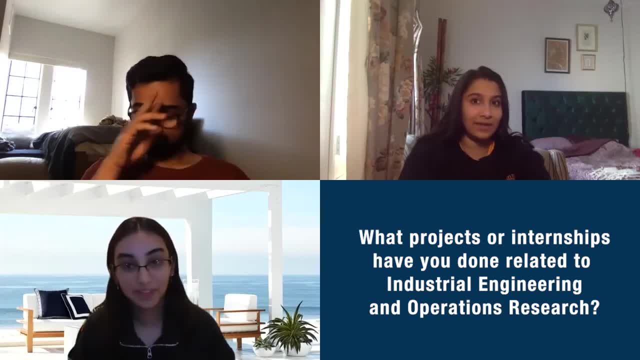 I've been in a lot of those companies, really kind of gone into depth in the IR department. also, kind of in the research space I'm currently working with Professor Anil Aswani on the bias and machine learning research And so through that I've kind of been learning how to like apply these different regression models. 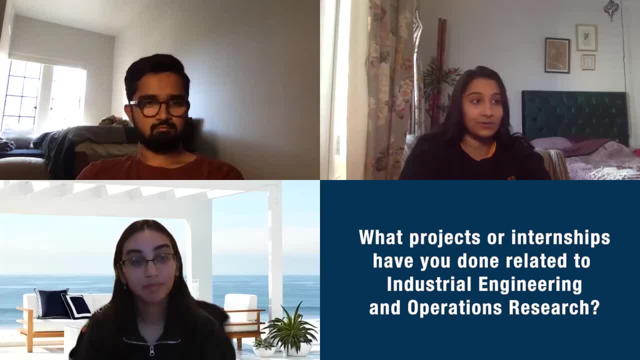 and understanding how to detect the bias and different algorithms through that And I think that's been super interesting. And then also along the lines of like entrepreneurship, I think I was really able to find different types of resources to start working on an idea with a couple other MET students. 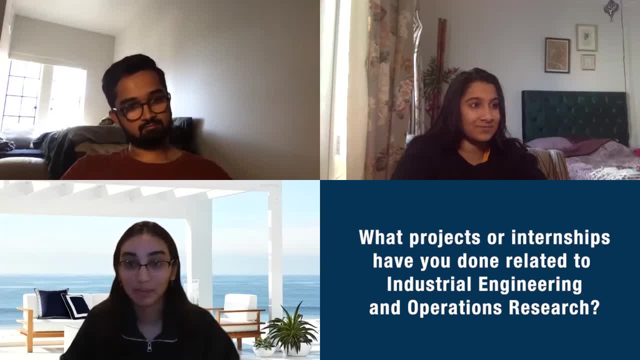 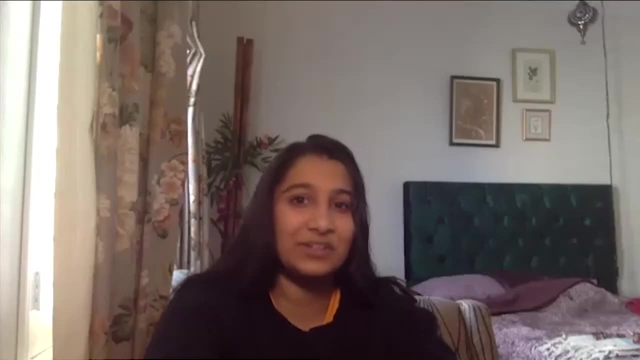 The IOR department is actually like, I guess, like the parent department of the Siddhartha Center of Entrepreneurship and Technology, And they offer a lot of classes through the department for entrepreneurship, So I definitely recommend checking them out. Last question: So what do you guys plan on doing with your major post grad? So I think I'm going to be doing a lot of things. I'm going to be doing a lot of things. So I'm going to be doing a lot of things. I'm going to be doing a lot of things. I'm going to be doing a lot of things.